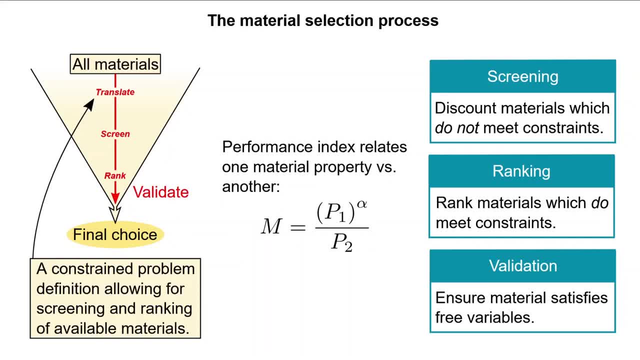 and is the critical thing which is required for these subsequent steps. It typically takes on the form of one property- P1, in this case raised to some power alpha, divided by another property, P2.. In an earlier example, the value of alpha was 1.. However, there are other translated use cases. 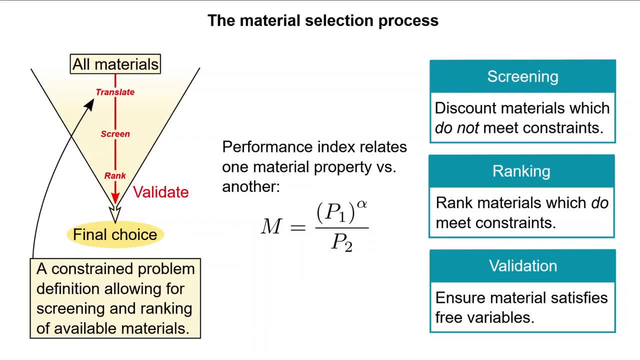 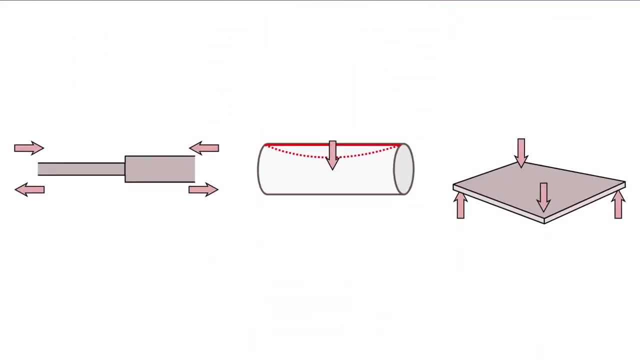 where alpha is not equal to 1.. Let's now look at some of those. We've already seen the performance index for a simple tie and you might have already seen the derivation of performance index for the deflection of a beam in the center here. 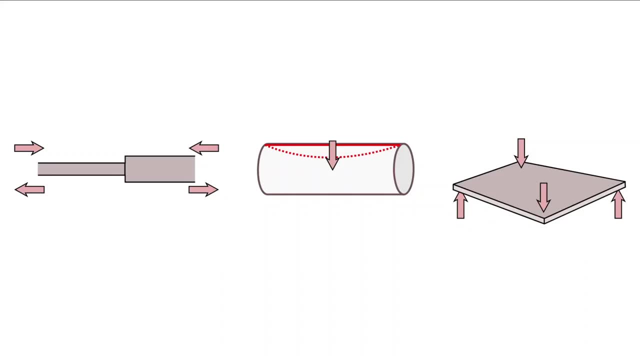 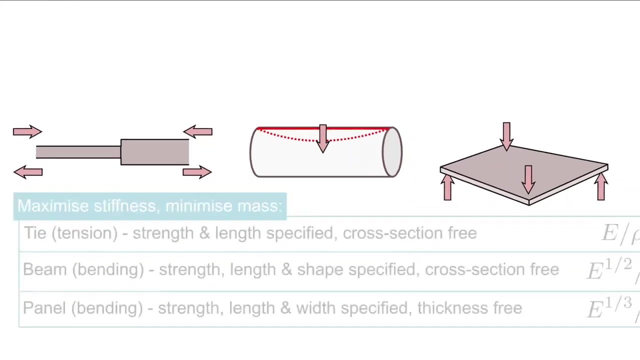 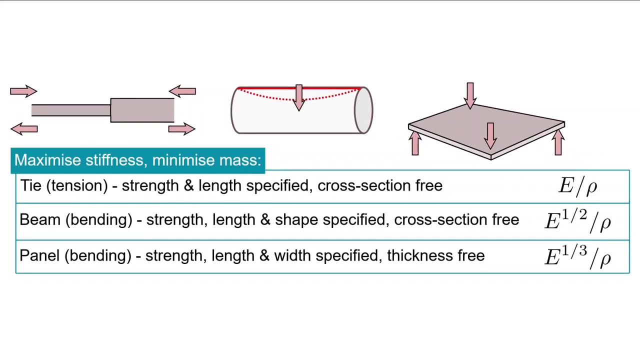 The performance index for the bending of a panel can also be derived in similar manners. For many engineering applications, making very stiff components that is resistant to deflection or elastic deformation is desirable, as is minimizing mass. The performance indices associated with maximizing stiffness while minimizing mass is given below for: 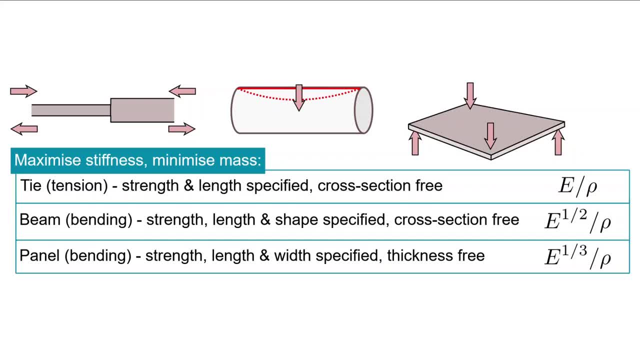 each of the types of the components described above. These are applicable on the basis of their strengths, and the performance index for bending of a panel can also be derived in similar manners, As well as some of their geometries being set, Relating these back to the original general form of the performance index. 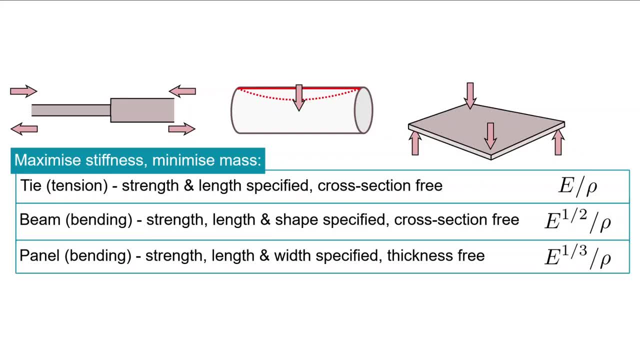 P1. here is the modulus of elasticity. P2 is the density and alpha ranges between 1 for a tie through to 1 half for a beam and 1 third for a panel, on the basis, again, of strength being defined. 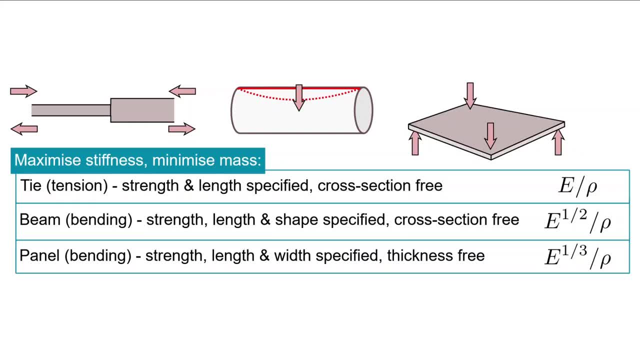 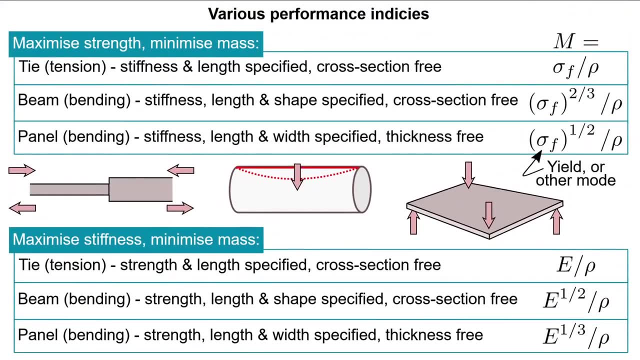 What if strength mattered instead, with the modulus fixed? Well, if the modulus is fixed, then the stiffness 2, is fixed on the basis of geometry To maximize strength and minimize mass. then these performance indices are used for each of the components described. 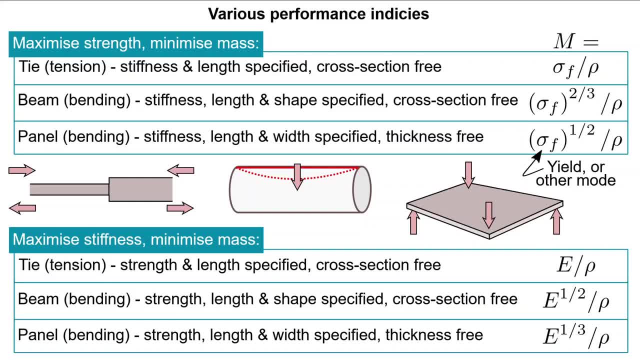 It's still P1, raised to some power, divided by P2, but P1 is now a failure. stress in order to be a broader descriptor, beyond the yield strength to account for all material forms, The values of alpha change, whereby it ranges from 1 to 2 thirds to 1 half. 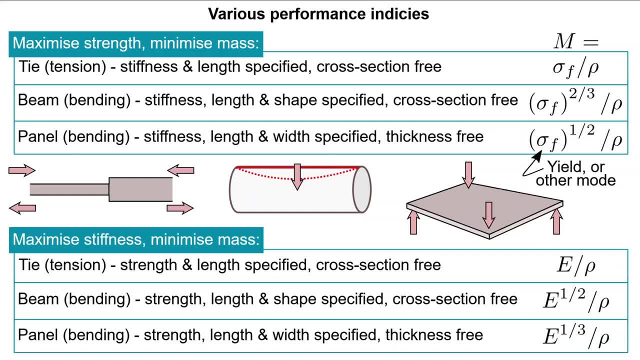 This is down to the relative differences in cross-sections for each of the parts. Complete derivations of the tie and beam are available elsewhere. Let's go ahead and apply one of the performance indices associated with maximizing stiffness while minimizing mass. Here's a simplified logarithmic plot of elastic modulus versus density. 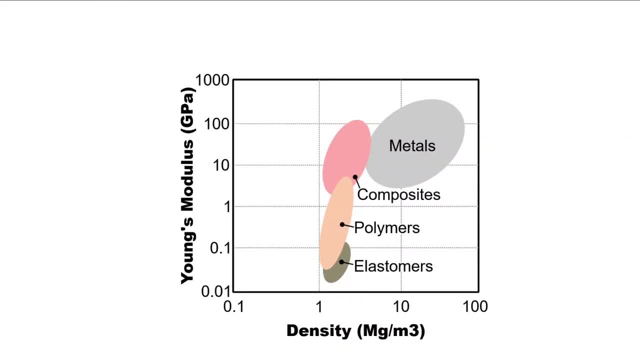 For most material systems that we've talked about in this course, The bubbles encompass all potential properties and may not be populated everywhere with specific materials. These few bubbles can, however, encompass hundreds, if not thousands, of different materials. We may plot our performance indices pretty much anywhere on this plot, as long as they have the correct slope. 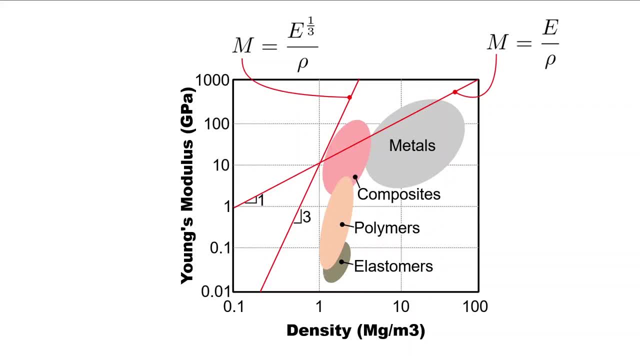 For example, a slope of 1 for a simple linear relationship between elastic modulus and density can be drawn anywhere. So too can a line corresponding to a panel. It will need to have a slope of 3,. however, The same is true for a beam. 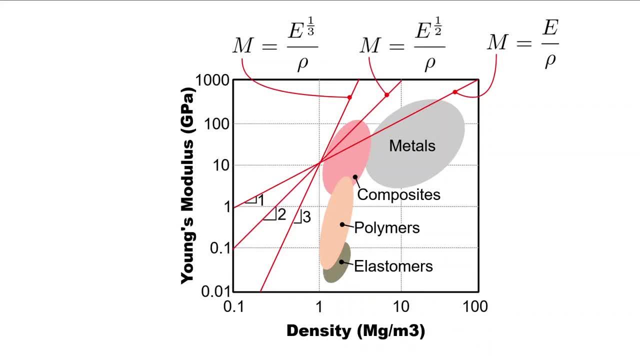 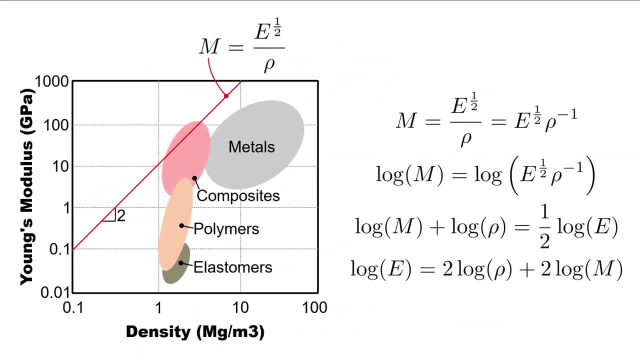 We can draw a line anywhere on the plot corresponding to this index, as long as it has a slope of 2.. Let's look at why that is. Using our performance index for a beam, we can break down the steps and meaning behind drawing this construction line. 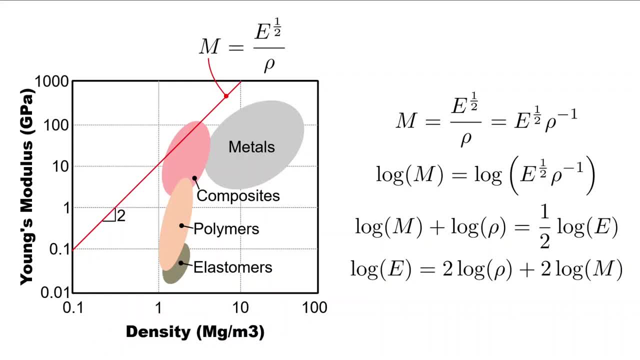 Rearranging the expression for the performance index. one takes the logarithm of both sides and isolates the logarithmic expression of the modulus of elasticity, which is dependent on the density and the performance index. From this manipulation you should be able to observe: 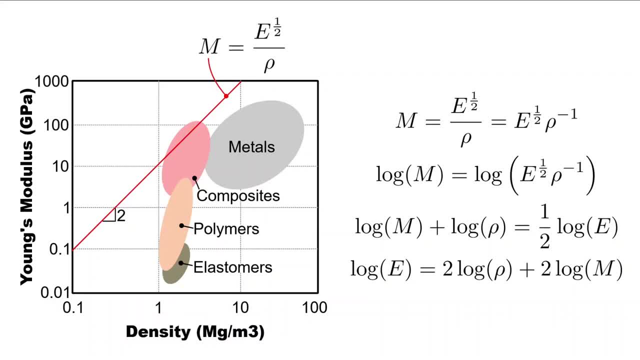 how the factor of two comes from the one half. This is the expression which is being plotted here. It has a slope of two which describes the relationship between modulus and density, and has an intercept of two times the logarithm of the index. However, if unconstrained, 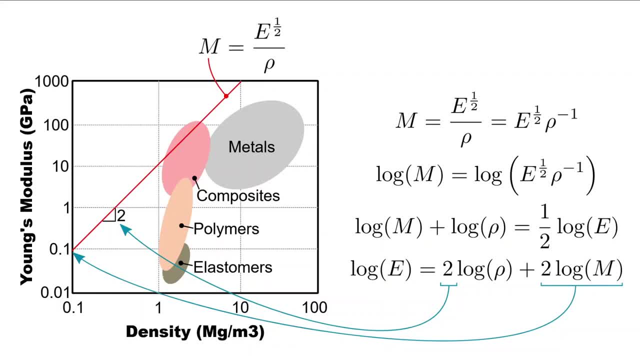 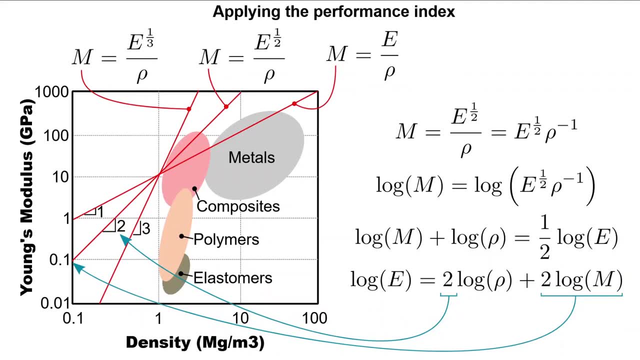 the index can change, which means that the construction line on this plot is free to move vertically along the y-axis. This is how one applies the performance index. You can see that for a given density, say one megagram per cubic meter, and a given modulus, there are no materials that are suitable for a given application. 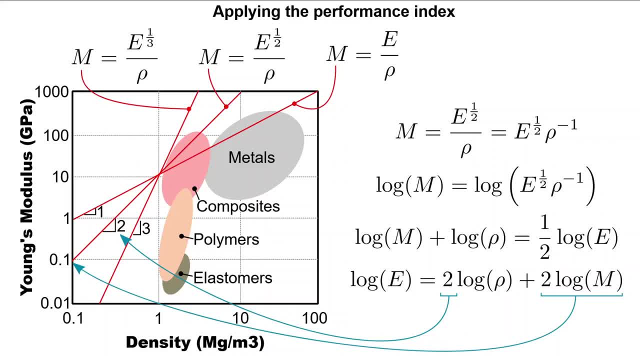 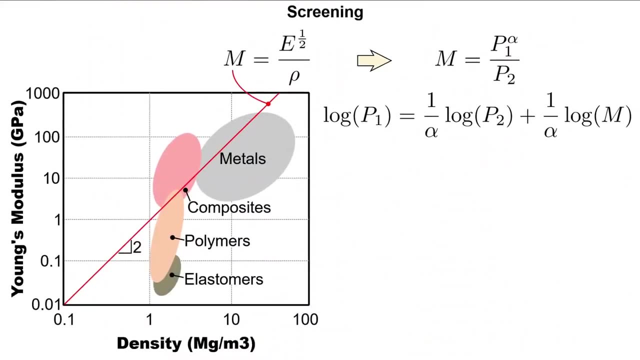 For a tie, one needs to increase the density by a certain amount before suitable materials are available, and similar conclusions can be drawn for the other component configurations and their respective performance index. We are now in a position to start screening. If you know what the performance index is, then you can jump to the general form of this. 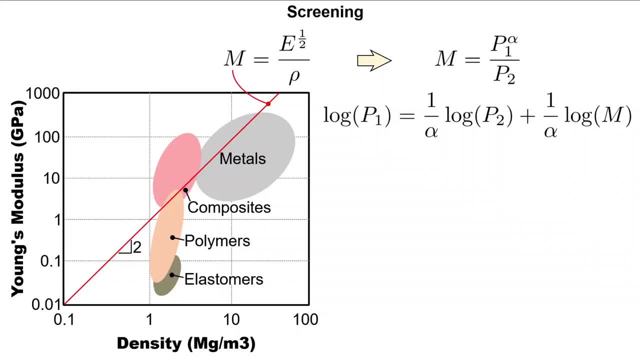 type of construction and set up for screening. Plotting the performance index alone in this manner does not uniquely identify any singular group of materials. All it does is identify a relationship between material properties. We need to apply some constraints that can be viewed in concert with this relationship. 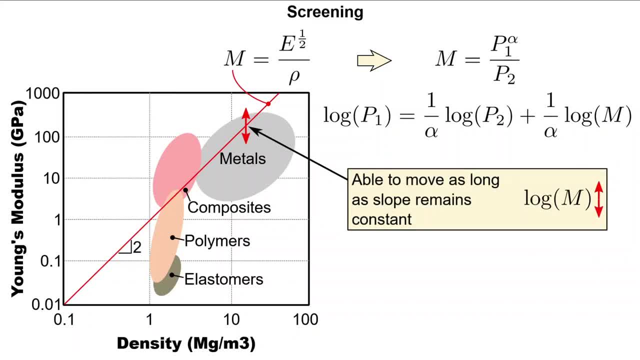 You can slide the performance index line up and down and you can draw it anywhere As long as it retains the same slope. We can also apply a second line corresponding to one of our constraints, such as that which corresponds to a minimum elastic moddolus. This line can move up and down as well. 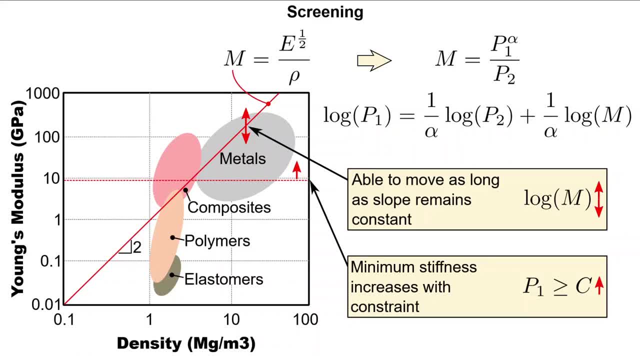 according to the constraint prescribed, but moves up as our minimum stiffness increases. The combination of both the performance index and the constraint now defines a search area. This search area now allows us to disallow or screen materials which are not suitable for the application. The constraint identifies a minimum stiffness and provides a lower bound. 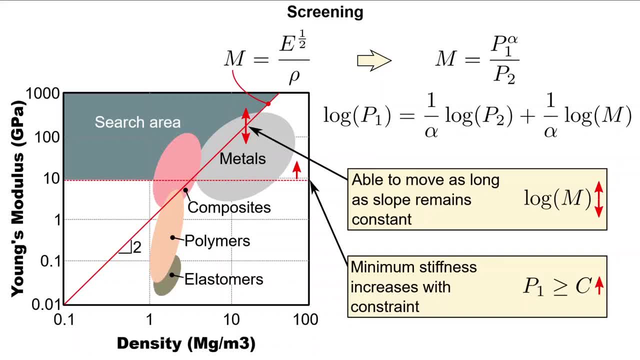 However, since the performance index is free to move, it does not identify material with a minimum density. This is why we need to rank our materials which appear in our search area. Say that we have only identified four materials that are available to us. 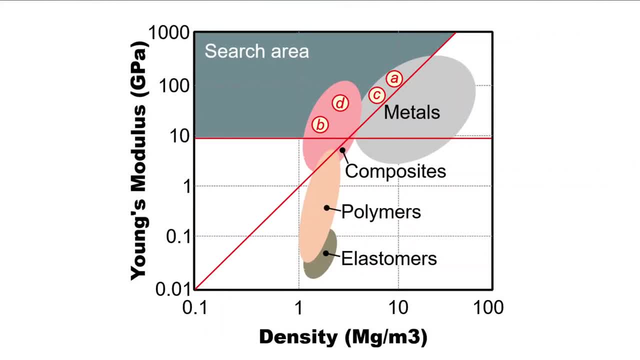 Remember, these bubbles corresponding to the varying material classes can contain many, many materials which may or may not be available, so this may be a realistic scenario. The performance index line can be shifted to include all four for consideration, such that the source is the same as the value of the material. The performance index line can be shifted to include all four for consideration, such that the source is the same as the value of the material. The performance index line can be shifted to include all four for consideration, such that the source is the same as the value of the material. 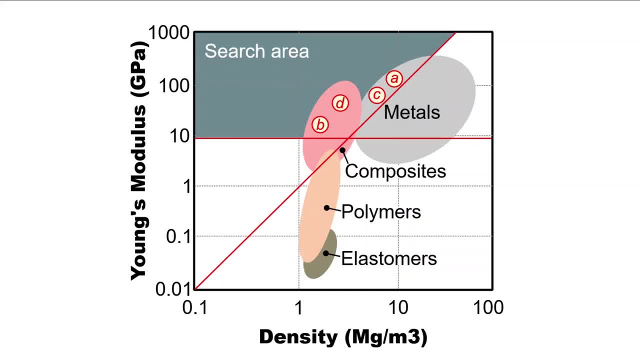 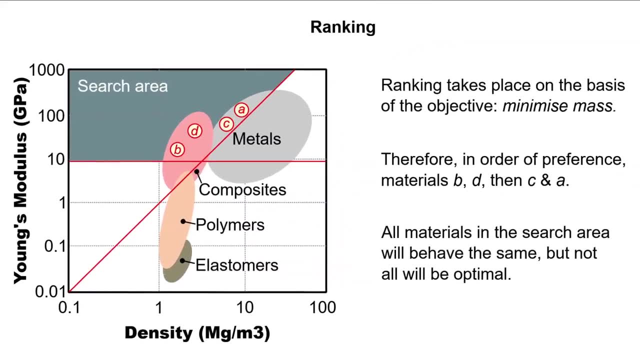 The search area contains the choices available. Two metals and two composites are to be considered. We go back to our objective for ranking which is the best choice. For the current example, this is to minimize mass. Therefore, on the basis of density, the best will be B, followed by D, C and then A. 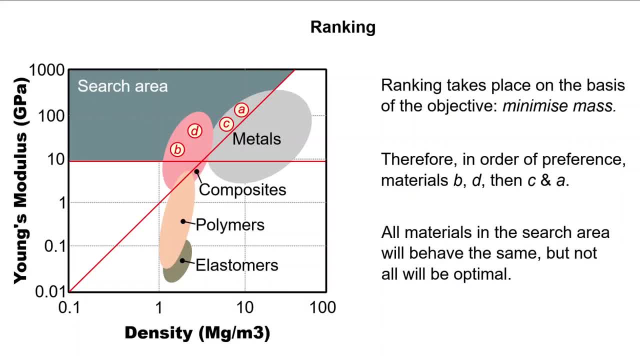 If the objective, and not constraint, is to maximize stiffness, then the ranking would run the other way, with A being the best choice, down to B. All the materials which are constrained in the search area will have the same relationship between modulus and density corresponding to a minimum acceptable modulus. 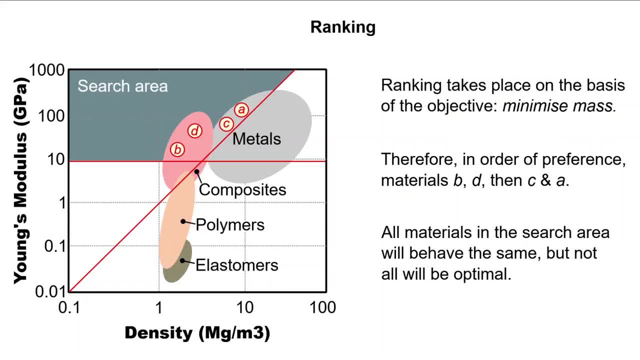 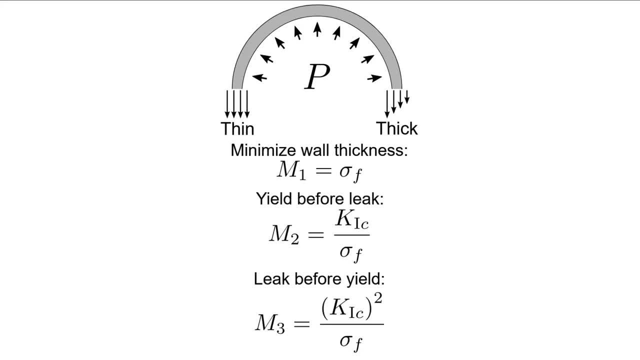 What happens if we need to consider multiple performance indices? If you recall the basics of pressure vessels from an earlier lecture, there are three main performance indices that can be employed when selecting a material for them. If one wishes to minimize the wall thickness of a pressure vessel regardless of flaws, 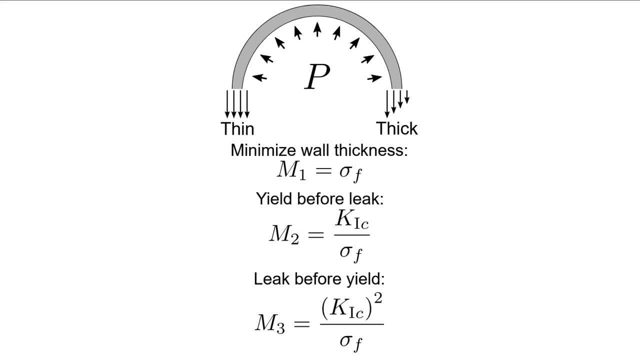 then the performance index is simply down to the failure or yield strength described by M1. If one wishes the pressure vessel to yield before it leaks, that is, the failure mode will be plasticity and not fracture. then a second performance index is a linear one. 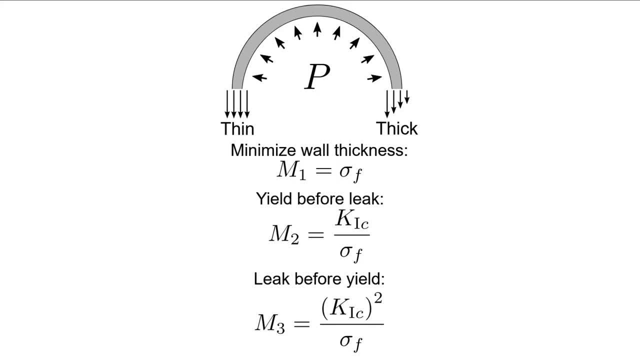 as described by M2.. Finally, If one wants the failure mode to be decided by fracture as opposed to plasticity, then M3 applies. There are design rationales behind each of these. For some, pressure vessels leaking will rapidly decrease the internal pressure and therefore 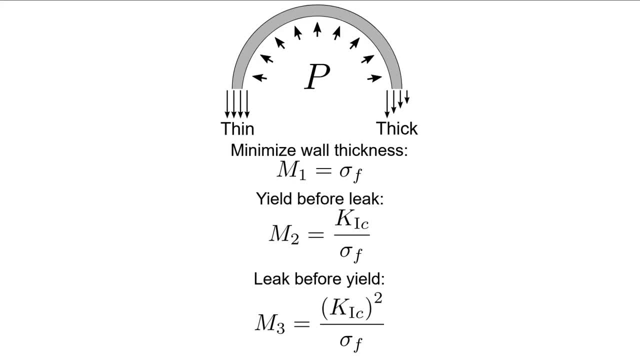 be less deleterious than failing by global plasticity. However, if the consequence of a leak will be worse than the vessel failing by plasticity, well, you get the idea. However, with our performance indices, we can actually apply all three. 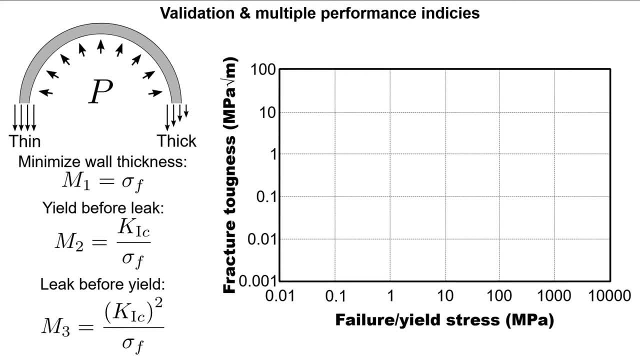 Plotting the logarithmic relationship between fracture toughness and the failure or yield stress. we can apply the same approaches as before, Starting first with M1, having a yield strength greater than a particular value, all of the materials that correspond to this. Next, we can apply M2.. 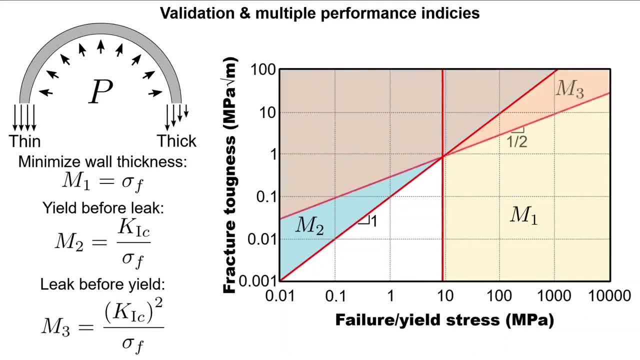 This further constrains the material choices. Finally, we can apply M3. M3.. In the locus where the label M3 is located, it can be seen that there is a conflict between M2 and M3. For the parameters given, M3 is more permissive than M2.. 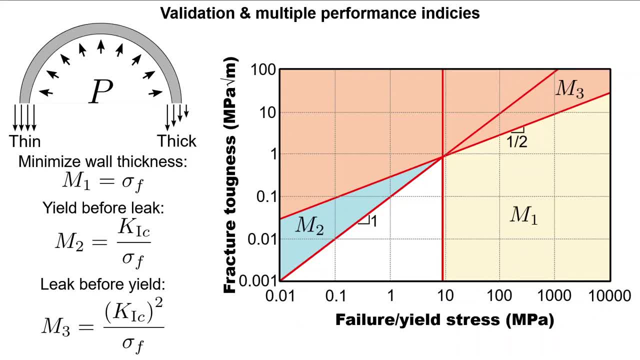 That is for a failure stress of approximately 10 MPa and a fracture toughness of 1 MPa root meter. By juggling all of these at once, we can arrive at both a framework for deciding which materials are best suited on a fracture properties basis, as well as minimizing wall thickness. 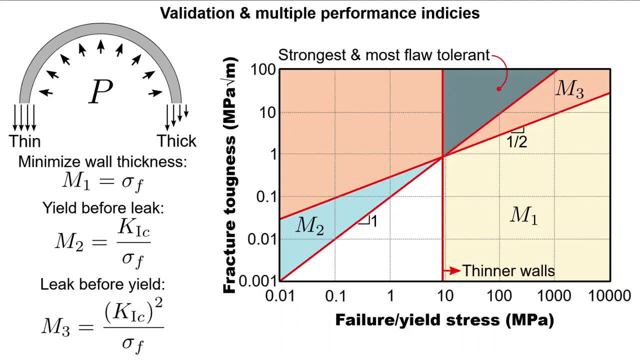 Furthermore, a potential locus of materials which can be employed to satisfy both yielding before leaking as well as leaking before yielding. which will be the strongest and the most flaw tolerant? We can then rank the materials according to which is more important: either yielding or 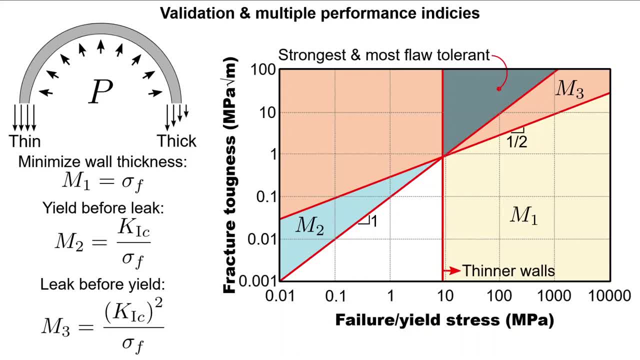 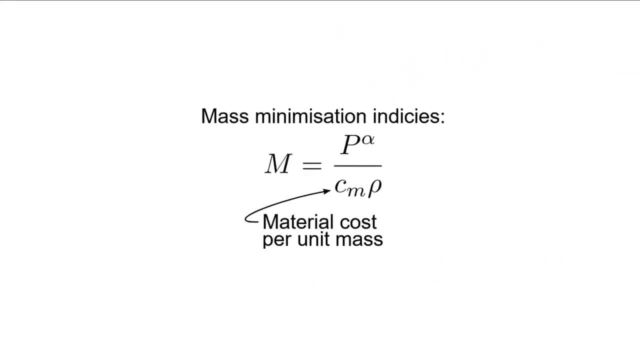 leaking. It might seem that this is the culmination of this entire approach, but there is one more step: Validation. 1., 2., 3., 4., 5., 6., 7., 8., 9.. 10., 11., 12., 13., 14., 15., 16., 17., 18., 19., 20., 21., 22., 23., 24., 25., 26.. 27., 28., 29., 30., 31., 32., 33., 34., 35., 36., 34., 35., 36., 36., 37., 38., 38.. 39., 39., 40., 41., 42., 42., 43., 44., 44., 45., 46., 46., 47., 48., 49., 50., 51.. 52., 52., 53., 54., 55., 56., 57., 58., 59., 60., 61., 62., 62., 63., 63., 64., 65.. 66., 67., 68., 67., 68., 69., 67., 68., 69., 69., 70., 71., 72., 72., 73., 73., 74.. 74., 75., 76., 77., 78., 78., 79., 79., 80., 80., 81., 81., 82., 82., 83., 82., 83.. 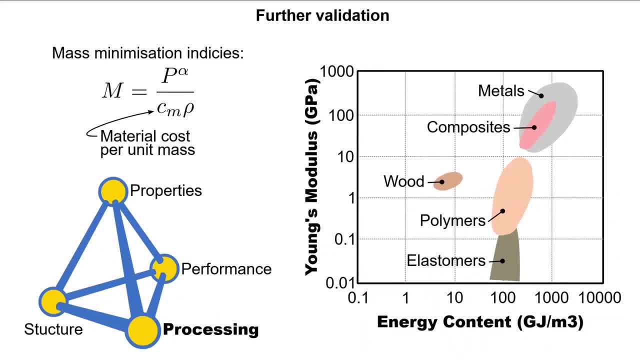 84., 84., 85., 86., 87., 86., 87., 88., 88., 89., 90., 99., 20., 21., 21., 22., 23.. 24. 25., 26., 27., 28., 29., 31., 31., 32., 33., 34., 35., 36., 36., 47., 38., 37.. 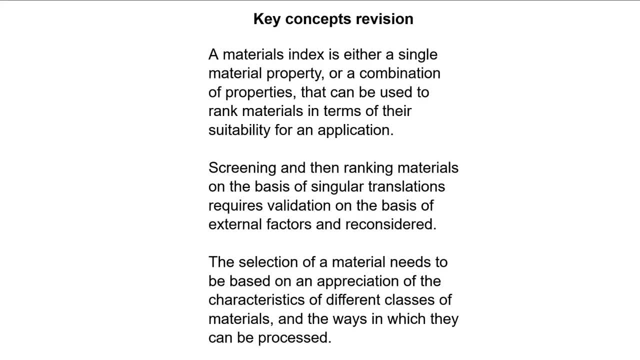 38., 39., 41. 42. performance indices at once has been presented. These indices, along with constraints to screen materials, ultimately validate down to a singular choice, And in choosing a material, you should now know a lot more about why materials have the properties that they do, both at the very small